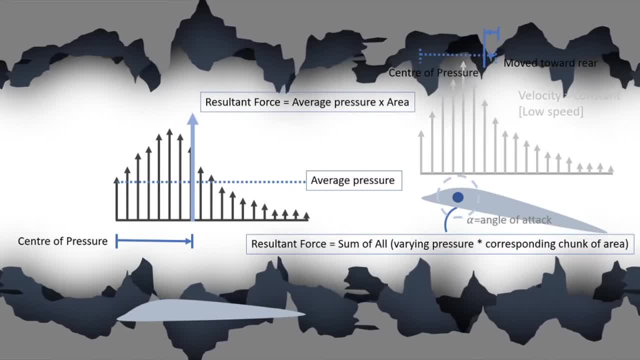 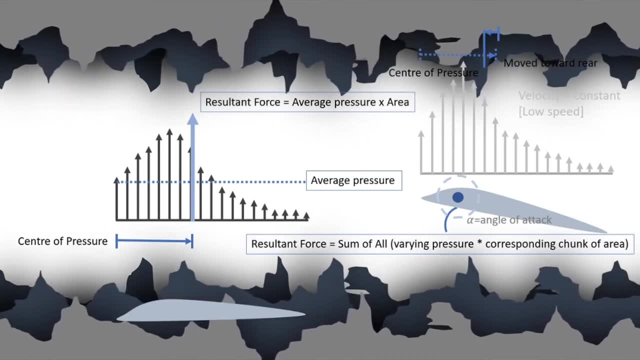 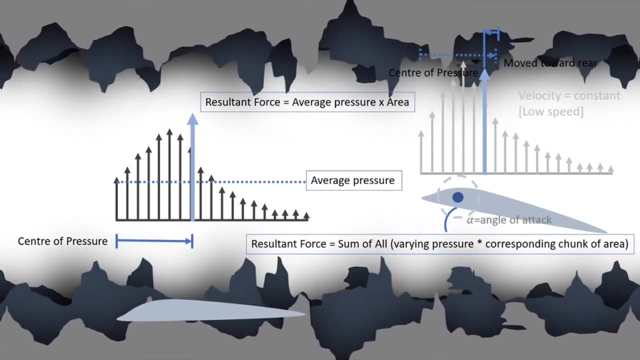 with the single resultant force at center of pressure. as you see in the second pressure distribution diagram, the center of pressure moves rearwards as the angle of attack increases. this might not move to rear in all cases. the moment of center of pressure with angle of attack is: 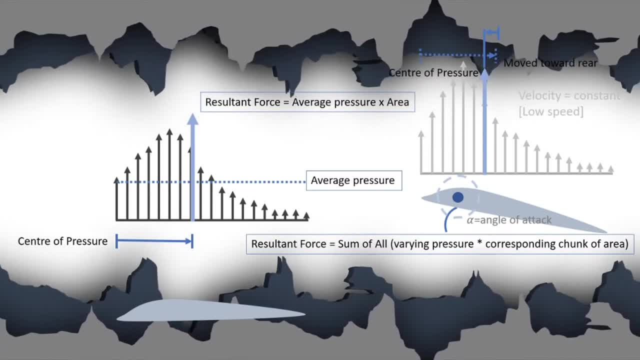 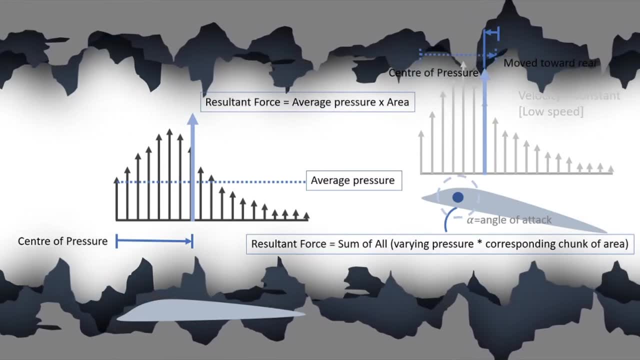 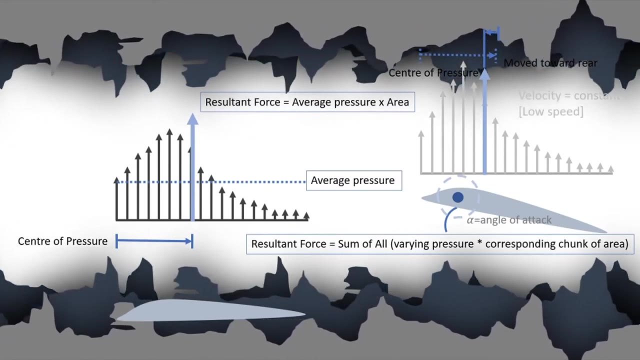 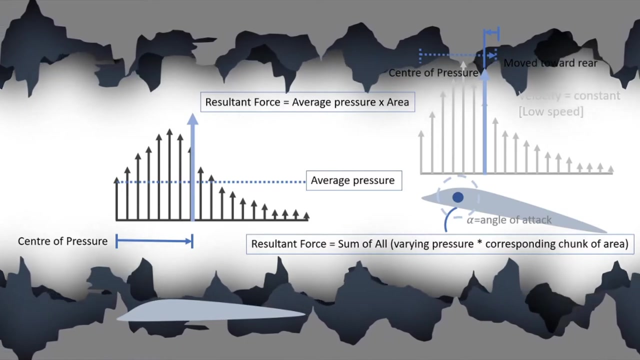 nonlinear and the moment varies depending on the airfoil design. okay, therefore, you cannot use center of pressure for most of the calculations. you need an another stable point for calculations. okay, before going to find that point at up, before going to find that point as a prerequisite, let us revise how to find the moment at one. 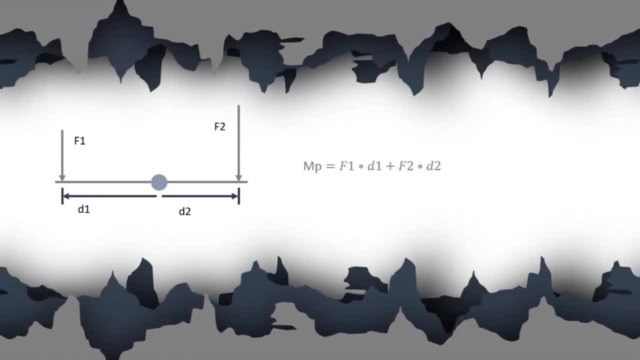 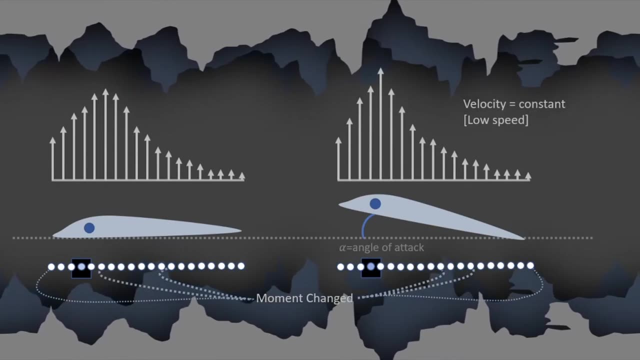 point moment at one point is the sum of all forces into the cross upon distance finding the movement. on each and every point on the cot, it is found that our 1-pointer is concerned for Georges Salah. and every point on that cot, it is found that at one point, this這是 concept lí subscribers. 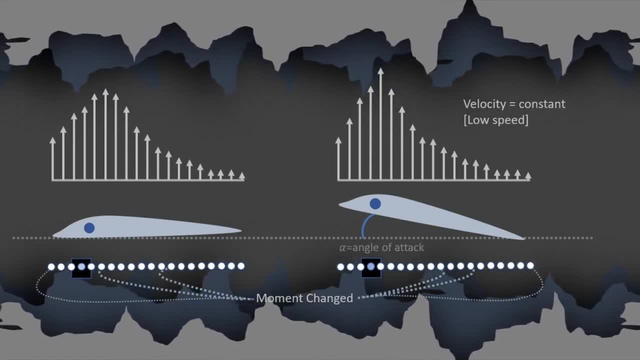 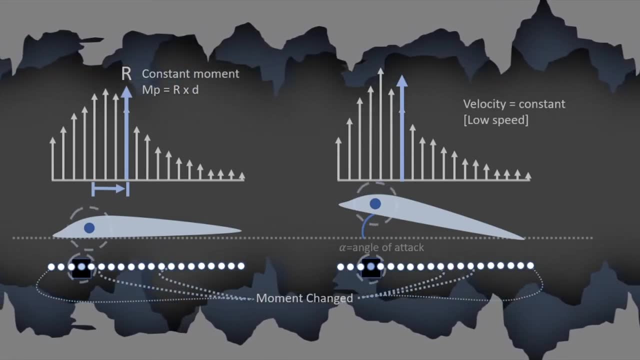 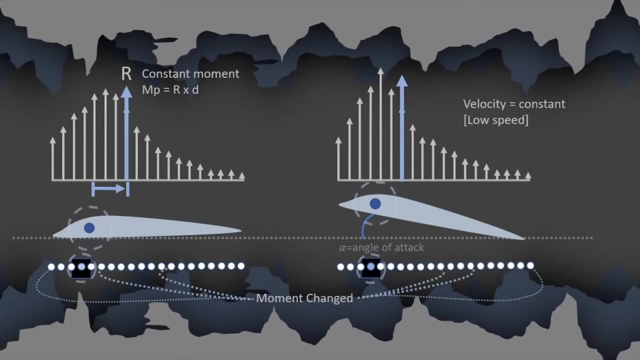 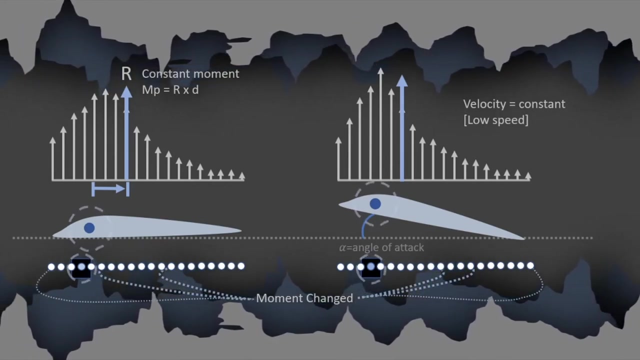 point: the movement generator remains constant, no matter what angle of attack is within the storm, and this point exists in airfoil by nature. this is the point called the aerodynamic center. very important to notice that it is valid only for the low speed- yes, at low speed- and also notice that the velocity is 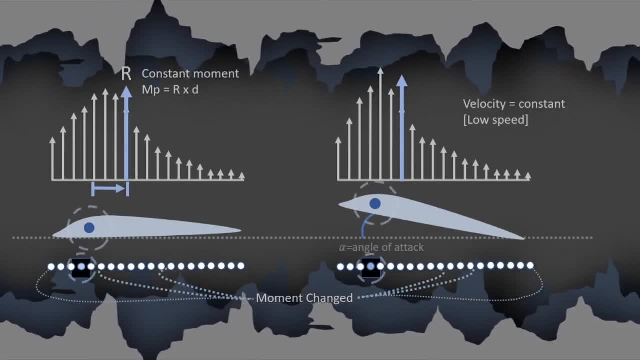 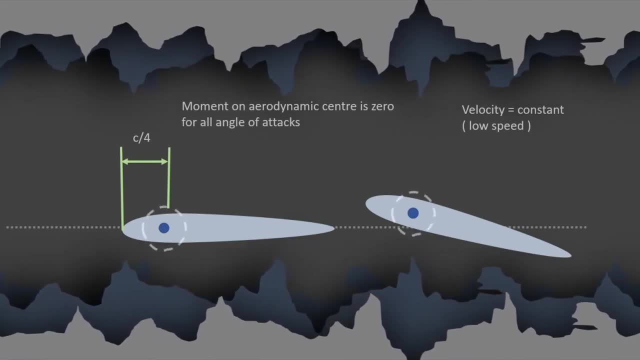 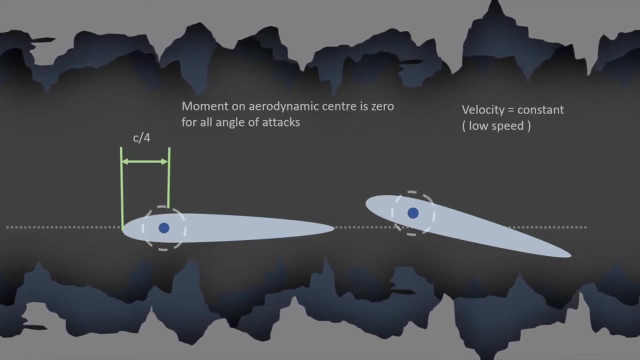 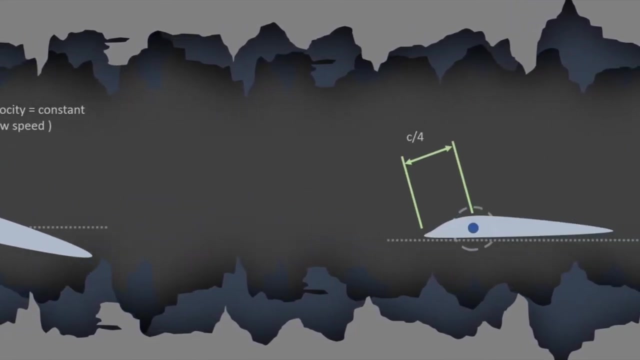 constant. theoretically, the aerodynamic center is located on the quad to quad on symmetrical airfoil. theoretically, the movement generated at the aerodynamic center is always zero. for a symmetrical airfoil, again, notice that it is valid only for low speed. for an unsymmetrical airfoil, the aerodynamic center is also located at 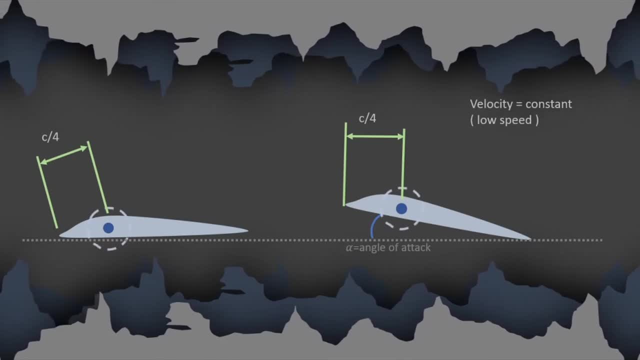 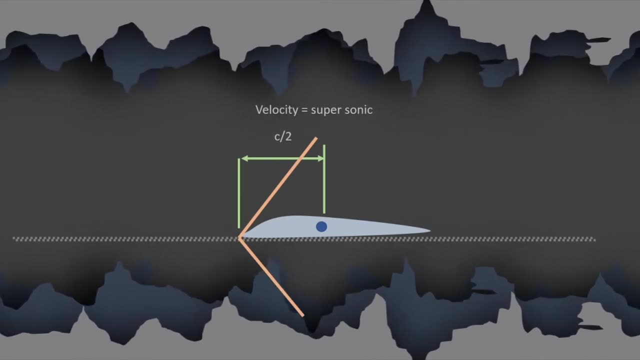 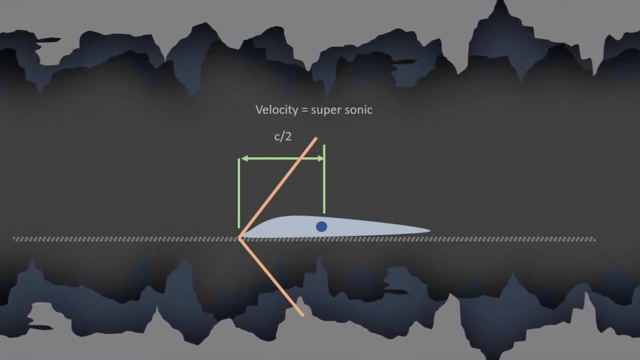 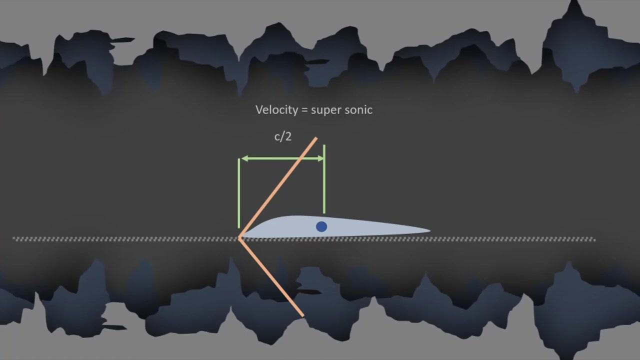 the quad to quad and the moment is constant, not zero. for supersonic flows, the aerodynamic center is located at half of the quad. probably you will not be using this value if you are designing a supersonic aircraft. you are going to find the aerodynamic center using CFD or experimental. but